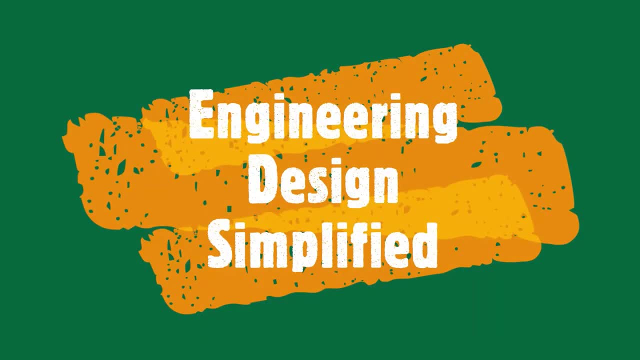 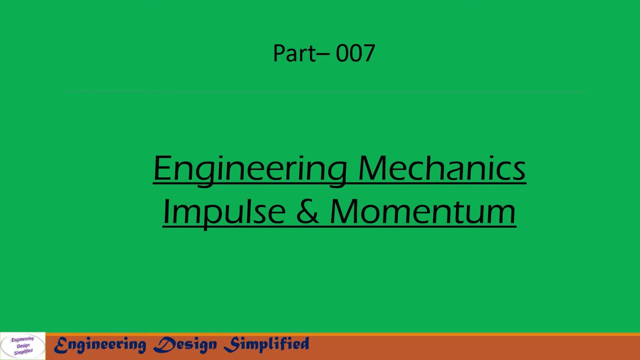 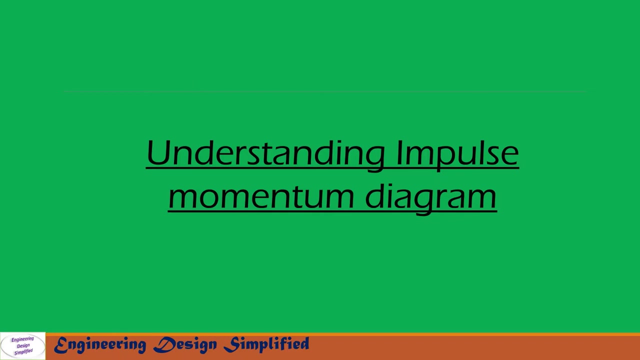 Hello engineers, welcome back to engineering design simplified. In this video series I will be solving tough engineering mechanics problems. If you want to watch more videos like this, please subscribe to my channel and press that bell button so that you will be notified when I upload a new video. In this video let us try to understand impulse momentum diagram. Let us assume 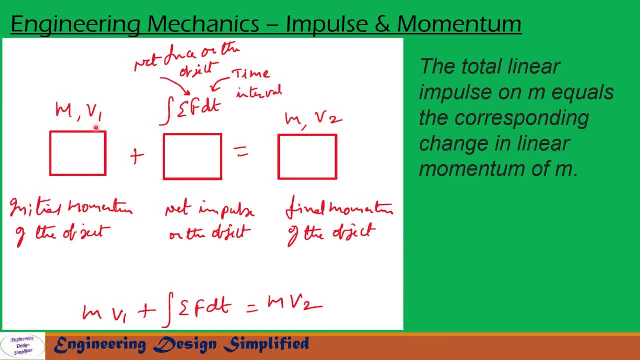 a body of mass m, and initially it is moving with a velocity v1.. So its initial momentum can be written as m into v1.. Now let us assume that there is a force- net force f- is acting for a time interval of dt, then the impulse on this object can be written as integral of sigma f into dt. 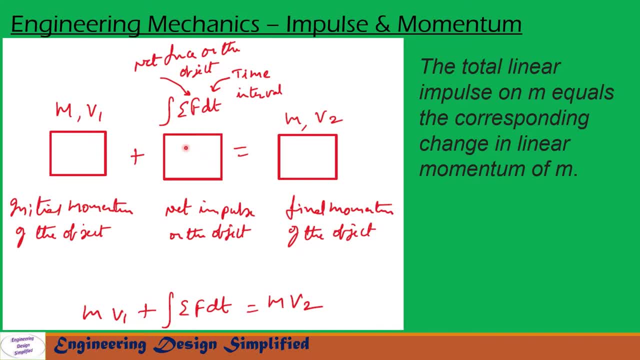 So when the force is applied on this body, on this moving body, then its final velocity will change to v2.. So its final momentum can be written as v1.. So let us assume that there is a force. net force can be written as m into v2.. So from this diagram we can write impulse momentum equation as: 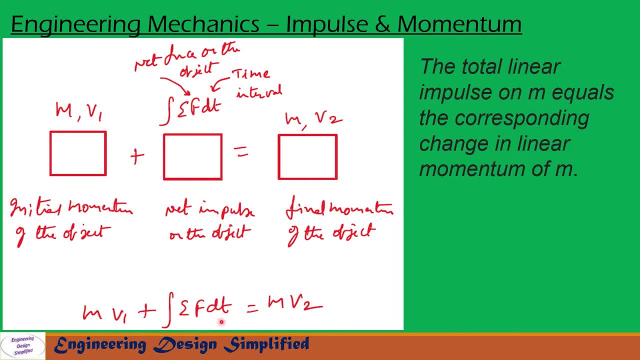 m into v1 plus integral of sigma f, dt equal to m into v2.. If we move this m1, mv1- that is the initial momentum- to right side of this equation, then right side of the equation will become m into v2 minus v1.. So this is the net change in linear momentum. So from this impulse momentum, 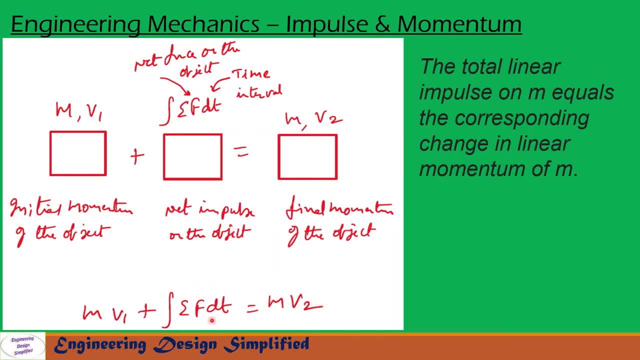 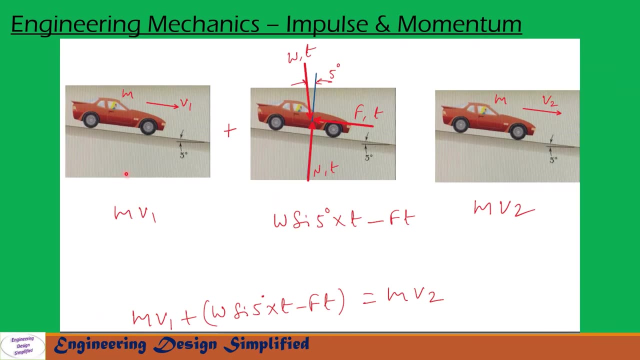 principle. so the total linear impulse on m on this object will be equal to net change in its momentum. So that is integral of sigma f, dt equal to m into v2 minus v1.. Now let us see an example here. a car of mass m or weight w is moving with a velocity v1 along this inclined plane. 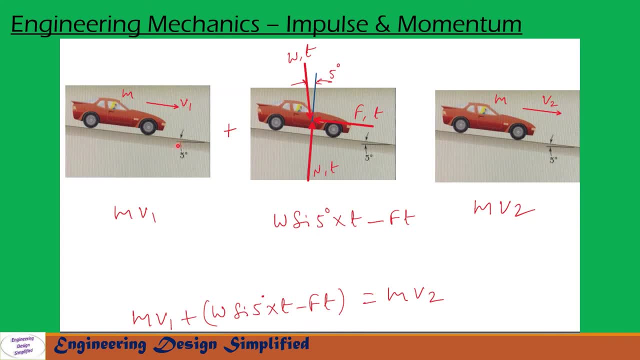 inclination is 5 degrees with a velocity v1.. So the initial momentum of the car can be written as m into v1 along this plane. Now when brakes are applied, then a force- braking force will oppose this motion of this body and weight is acting vertically downwards and a normal reaction n.